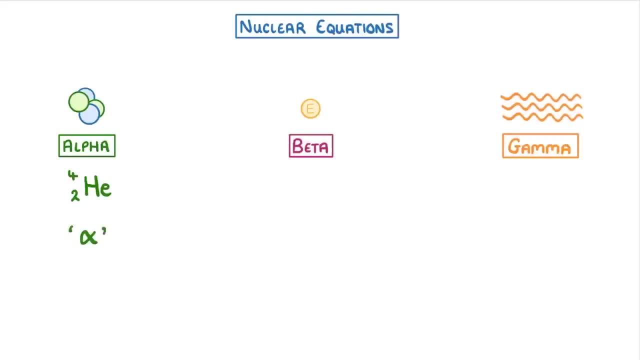 might sometimes see them as the Greek letter alpha instead. So when an unstable nucleus like uranium-2,3,8, undergoes alpha decay and emits one of these alpha particles, it's going to lose two protons and two neutrons. To show this, we 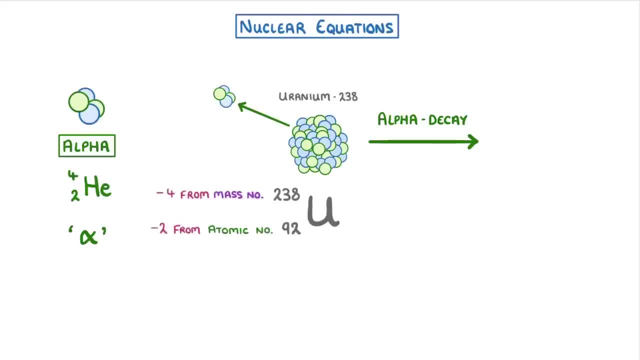 have to subtract 4 from its mass number and 2 from its atomic number, So uranium-2,3,8 would go to form something like this: Something with a mass number of 2,3,4, and an atomic number of 90. Because the atomic 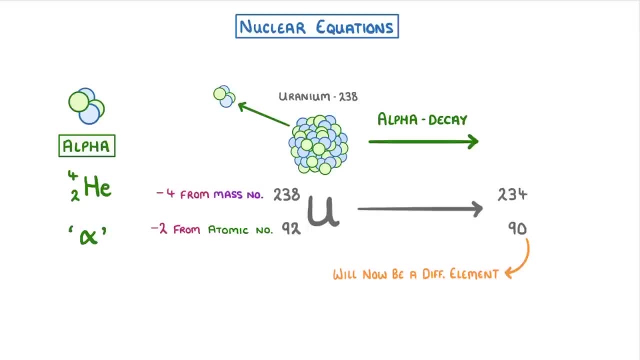 number has changed. it will now be a different element, So we'd have to check the periodic table to find out that it's now thorium. The last thing is to add our helium that was emitted and then just double check that the mass and atomic numbers on each side of the equation are the same overall. 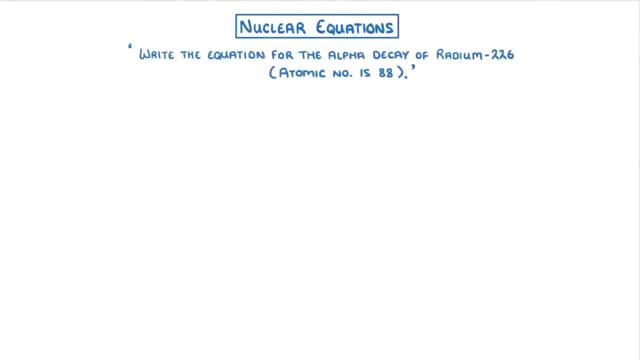 So if we had a question that asked us to write the equation for the alpha decay of radium-2,2,6,, which has an atomic number of 88,, we would start with our radium-2,2,6, and. 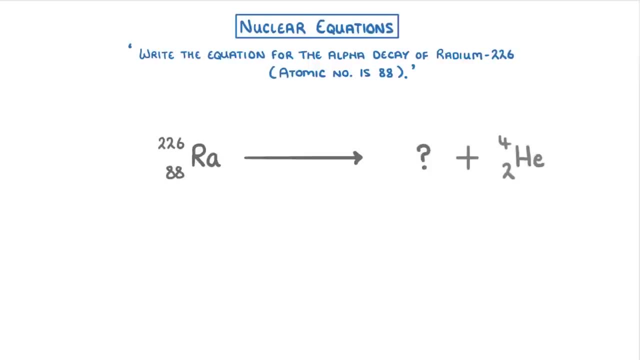 draw an arrow to our unknown decay product and our alpha particle, which we write as a helium nucleus. Then, to figure out what our decay product is, we subtract 4 from the 2,2,6 to get a mass number of 2,3,4, and then just double check that the mass number is. 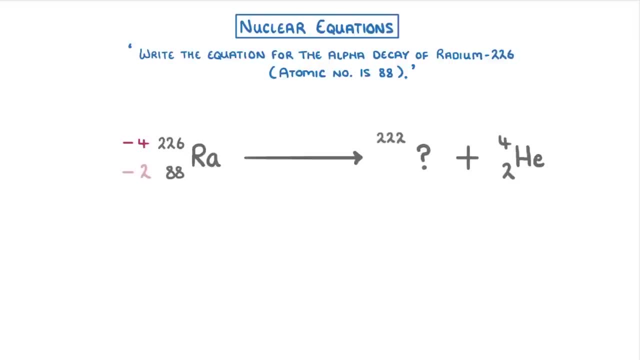 2,3,4, to get a mass number of 2,2,2, and minus 2 from the 88, to get an atomic number of 86. Then all we have to do is check the periodic table to figure out what element. 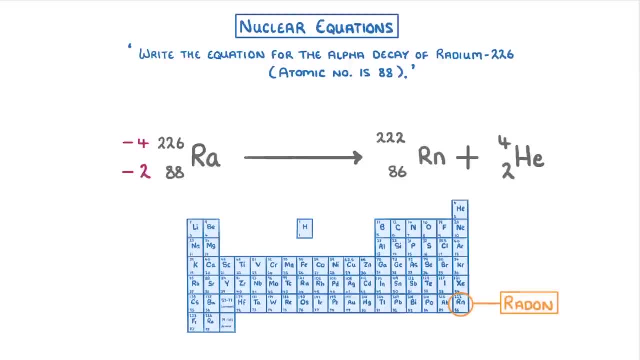 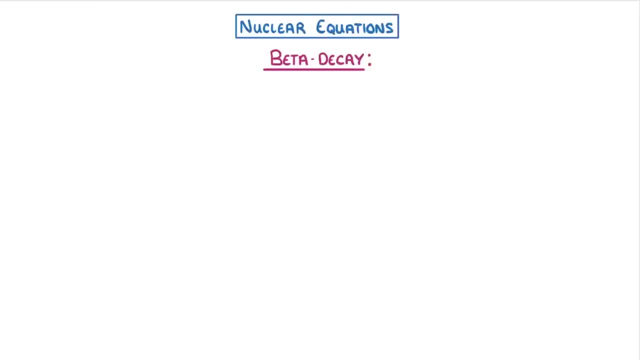 it is, So in this case, radon. Now, beta decay is a bit more complicated because it involves a neutron turning into a proton and emitting a fast moving electron. So if carbon-14 was to decay and emit one of these electrons, then because it's effectively 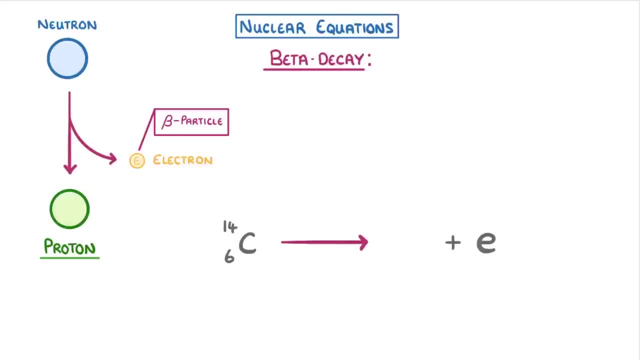 gained a proton, it's atomic number would increase from 6 to 7, making it nitrogen rather than carbon. However, it's mass number would stay the same because, although it's gained a proton, it also lost a neutron, so it still only has a total of 14 protons and neutrons.